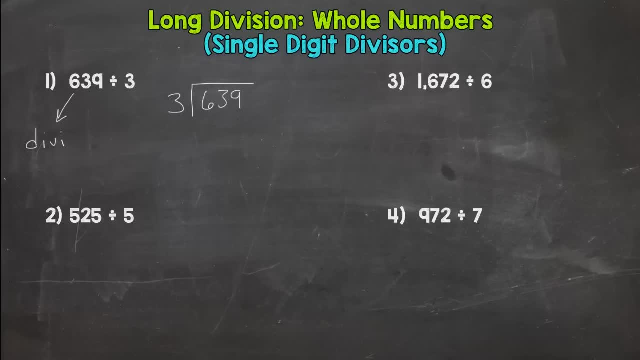 Here and I'll spell it out: D-I-V-I-D-E-N-D. Dividend, It's what we are splitting up, And then divisor is what we call that 3. It's how many groups we are dividing up. It's how many groups we are splitting 639 up into. 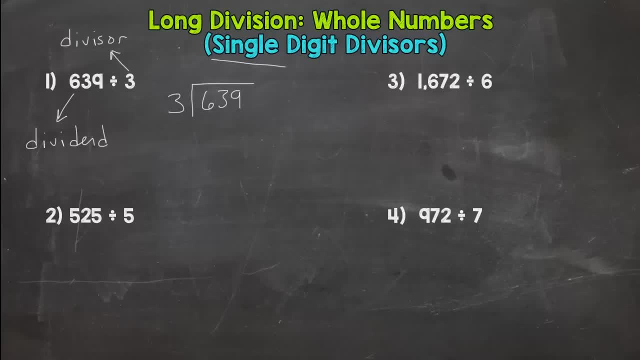 Okay, how many groups we are splitting it into. So single digit divisor is going to be. you know that outside number, All of these will have a single digit divisor. So the first thing we want to do when we have a long division problem is we want to divide. 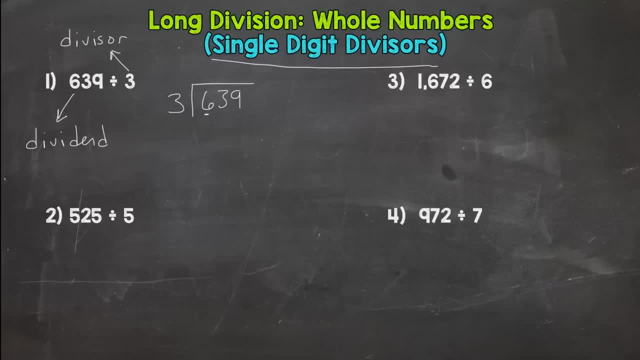 We look at the first number here in 639, the 6, and we ask ourselves: well, 6 divided by 3. How many groups of 3 can we pull out of 6?? And the answer is 2.. And then we multiply this 2 by the 3.. 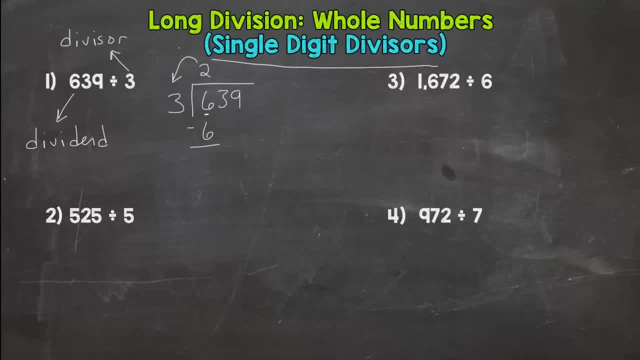 2 times 3 is 6.. Then we subtract 6 minus 6 is 0. And then we bring down and start that process over again. So our process was: divide, multiply, subtract, bring down. Sorry, my C in subtract looks like an O, That's a C though. 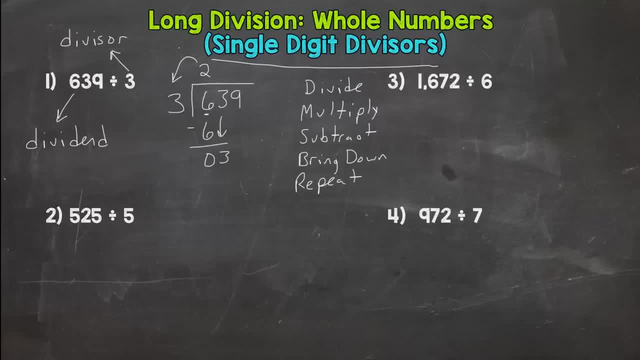 And then we repeat the process. So we are on the repeat step. So we need to do 3 divided by 3.. How many groups of 3 are in 3?? And the answer to that is 1.. Now we multiply. 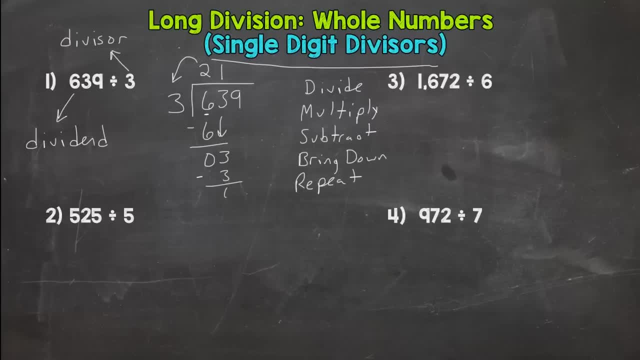 1 times 3 is 3.. Subtract We get 0. Bring down our 9. And then repeat, So 9 divided by 3. Or how many groups of 3 are in 9?? Well, 3,, 6,, 9,, 3.. 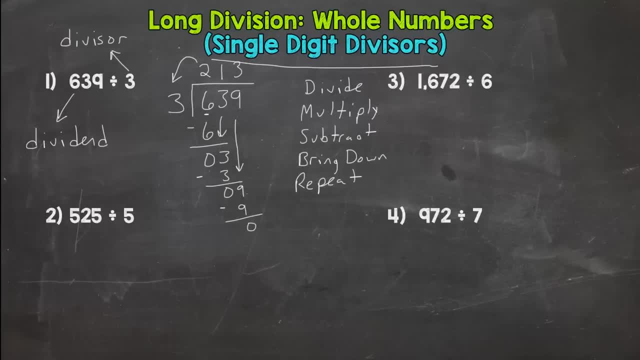 3 times 3 is 9.. Subtract And we get a 0.. Now we went all the way over to our lowest place value, which is the ones place, And we don't have anything left to bring down. And this 0 tells us remainder of 0. 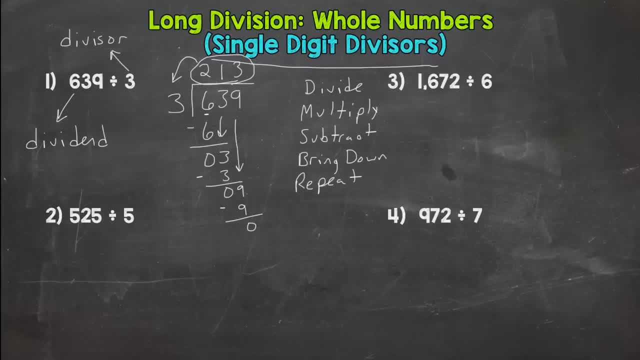 We are done. Our quotient is 213.. And quotient means answer to a division problem. Now, that might have seemed very confusing And a lot of people don't know that There are a lot of steps there, But just take a look at these steps when you get stuck. 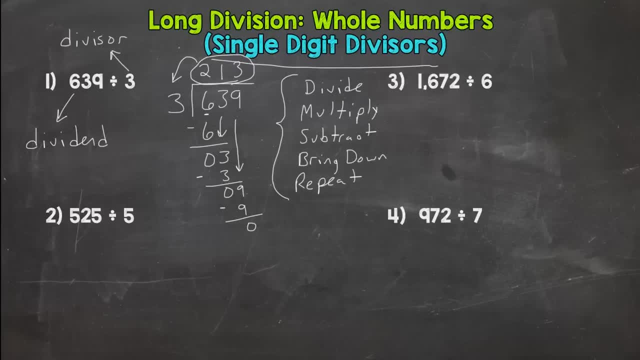 And you will get it down with practice. The biggest thing to mastering this is doing problems and practicing. So let's go to number 2.. 525 is our dividend And 5 is our divisor. Well, divide first. 5 divided by 5 is 1.. 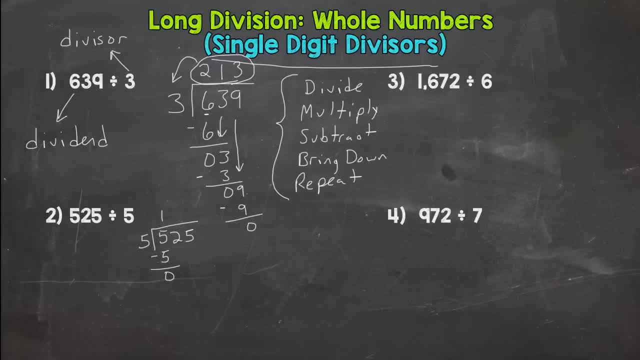 1 times 5 is 5. Subtract, Bring down. Now this is something a little different. here We have a 2 divided by 5. How many groups of 5 can we make or pull out of 2?? Well, we can't. 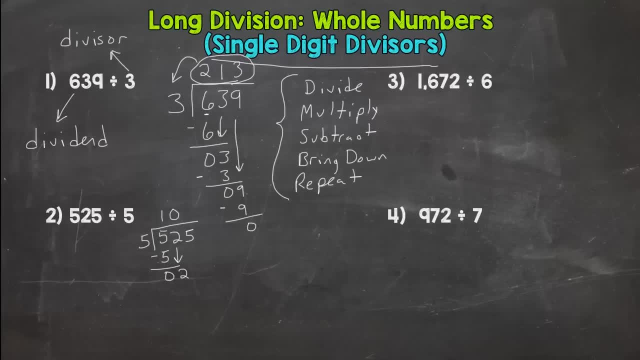 So we need to put a 0 here. 0 times 5 is 0.. Subtract: We get a 2. Bring down that: 5.. Now we have a 25.. 25 divided by 5 is 5.. 5 times 5 is 25.. 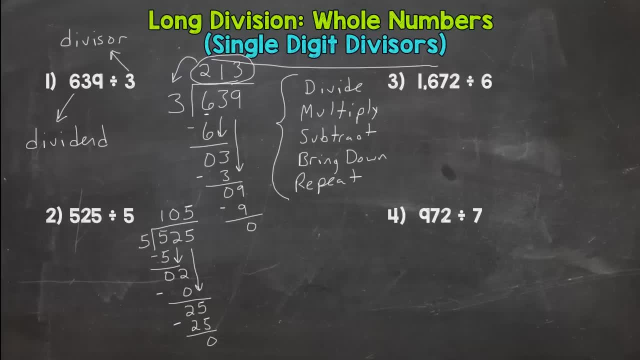 Subtract, We get 0. Went all the way over. Nothing else to bring down. 105 is our answer, with a remainder of 0. So number 3.. We have a 4 digit dividend and a single digit or 1 digit divisor. 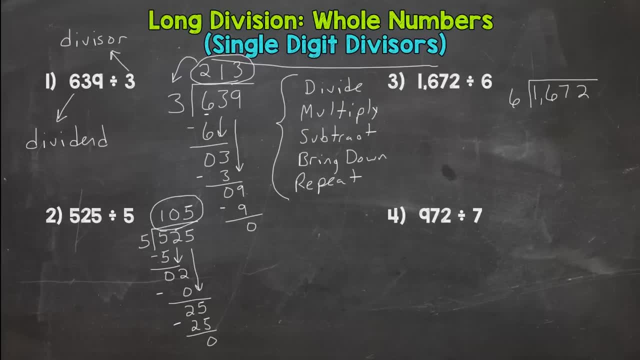 So let's look at the 1. here We need to do 1 divided by 6, which we cannot do. So we need to look at the 16.. How many groups of 6 can we pull out of 16? Well, 6.. 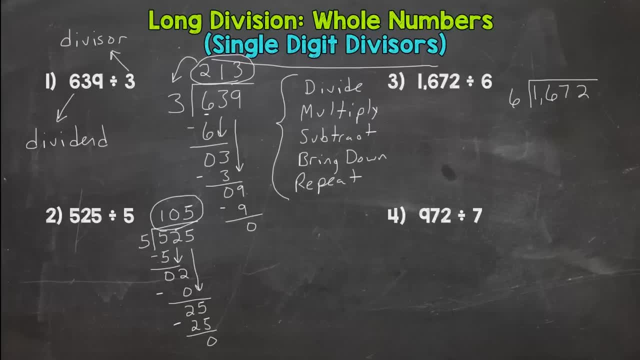 12. 18.. 3 was a 1.. 3 was too many, So it's just 2.. And the 2 needs to go above the 16. Not above the 1., Above the 16.. Everything needs to line up here. 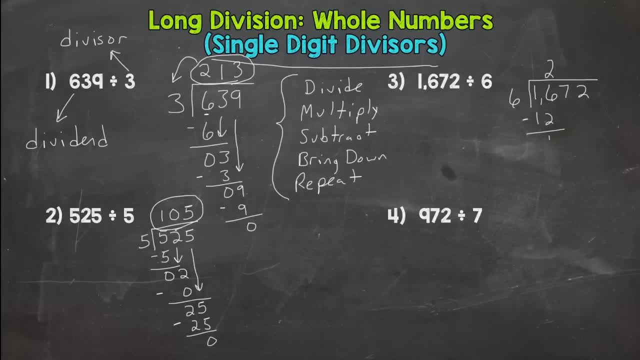 2 times 6 is 12.. Subtract We get 4.. Bring down the 7. How many groups of 6 out of 47?? So you have to think of your 6 multiplication facts or count up by 6's to get as close to. 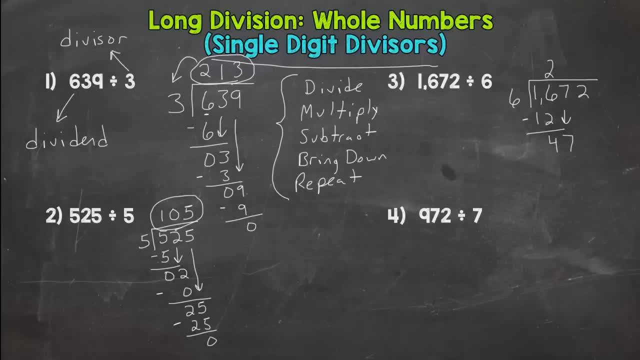 47 as you can without going over. So how many groups of 6 out of 47?? Well, 6 times 6 is 36.. 6 times 7 is 42.. 6 times 8 is 48.. 8 would be a little bit too high, so it's going to be a 7.. 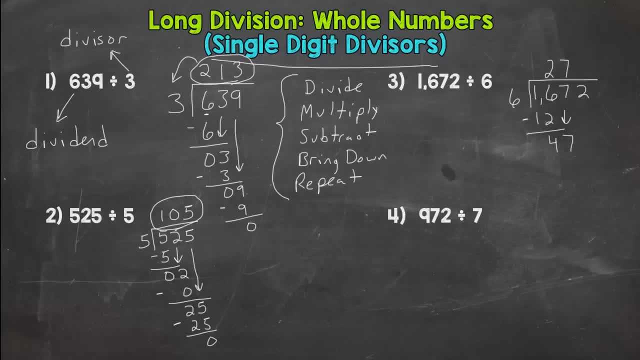 42 is as close as we can get. 7 times 6 is 42.. Subtract: we get 5.. Bring down the 2.. So 52 divided by 6.. Well, we just said, 6 times 8 is 48.. 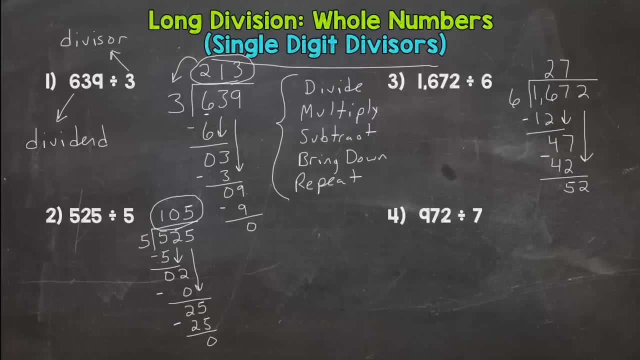 6 times 9 is 54.. Bring down the 2. 9 was too much, so it's an 8 here. 8 times 6 is 48.. Subtract, We're left with a 4.. Now, there's nothing left to bring down. We're all done with our process. This 4 down. there is what we. 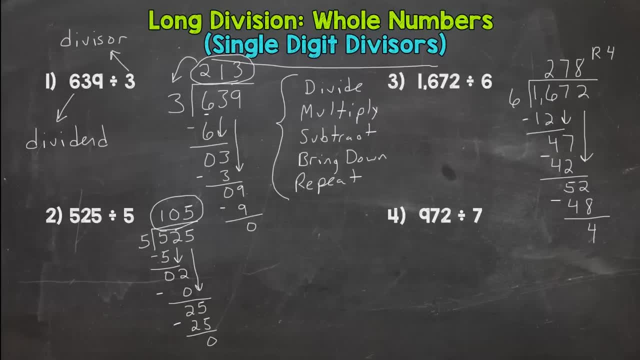 call the remainder. It is what is left over after we've split 1,672 into 6 groups. Each group will have 278, and then there's 4 left over. It didn't divide out perfectly into a whole number. 4 were. 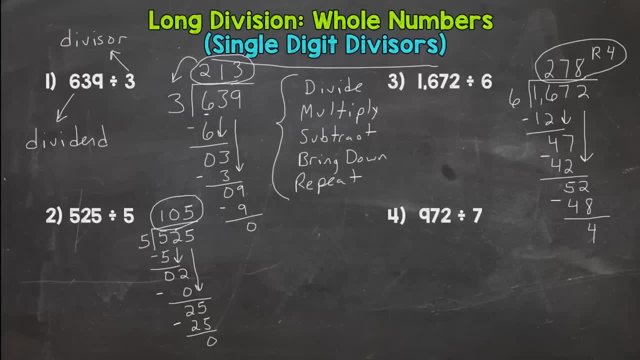 left over, and that's okay. Number 4,: 972 divided by 7.. So we start with 9 divided by 7.. How many groups of 7 are in 9?? Well, 1. 1 times 7 is 7.. Subtract We get 2.. Bring down the 7.. 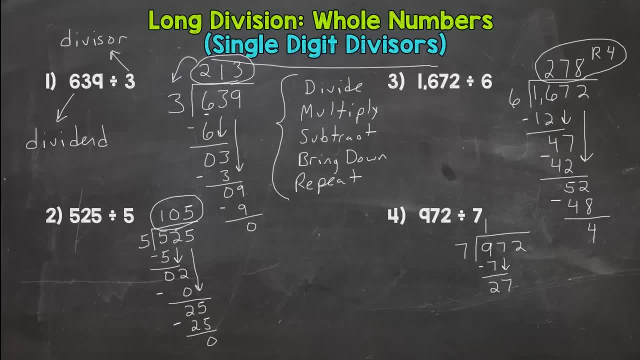 How many groups of 7 out of 27?? Well, 7,, 14,, 21,, 28.. 4, a little bit too many. so only 3: 7s. 3 times 7 is 21.. Subtract We get 6.. Bring down that 2.. So we have to think of our 7 facts. Well, 7 times 7, 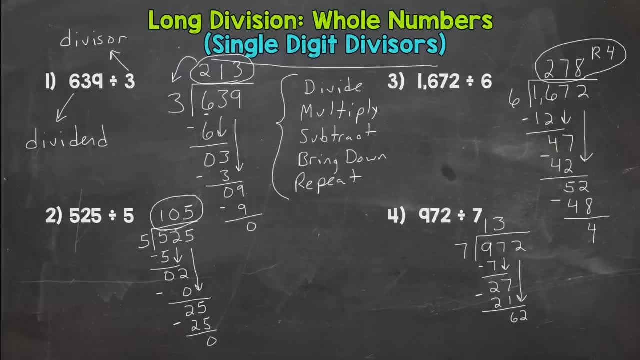 is 49,. but we can get a lot closer than that: 7 times 8, 56.. 7 times 9,, 63. So 8 is as close as we can get. 8 times 7 is 56. Subtract, We get a remainder of 6.. So 138,.